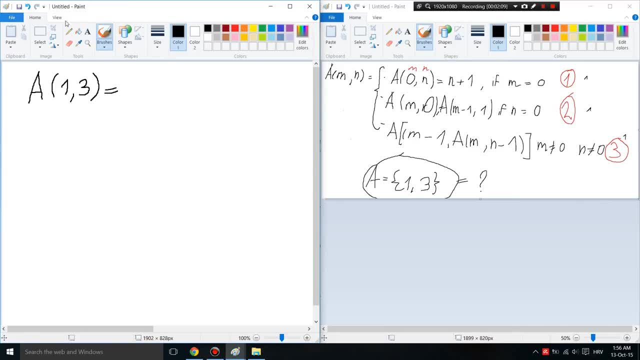 a tree. okay, so you have M and and, and M is one and n is three. so you go here and you look at the rules and you see that rule number three is: if M is not equal to zero and n is not equal to zero, then you subtract one from M and. 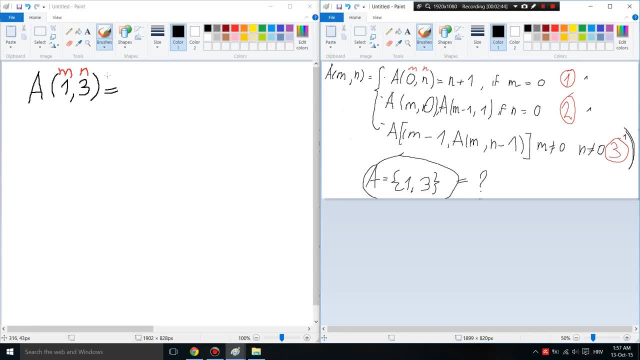 then okay, so it should look like one put the three, so now we're using three, so it should look like a subtract one minus one zero. and then we can use this, this one here, and we get one, two, because we subtract one from the tree, that's it. 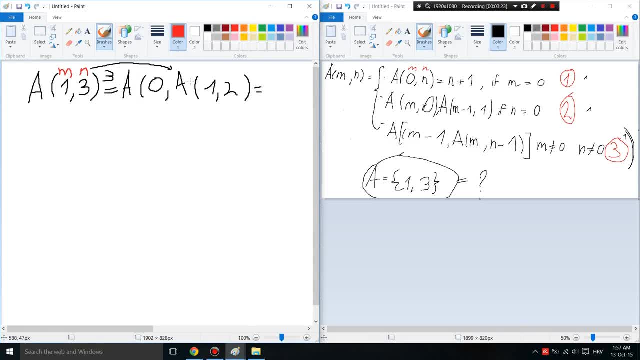 now you take this, you just place it down here. now you start again with a one, two. again, we're going to use number three and it's going to be a 0 Chelых, about a 0 Chelых and subtract one, you see from the end, and we're gonna get one one. 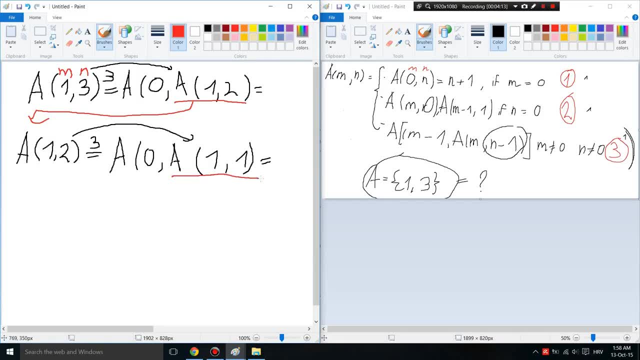 okay. so now you take this over here, you're okay. one one again. we're going to use rule number three and we get a zero and a one zero again because we subtract and hope it's clear, and then again we take this and we start from this zero. but now it's different rule, it's rule number two. 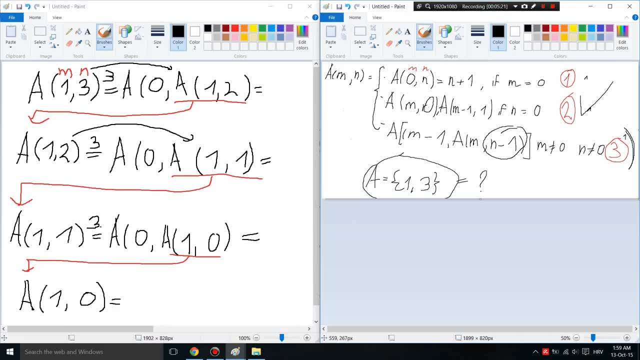 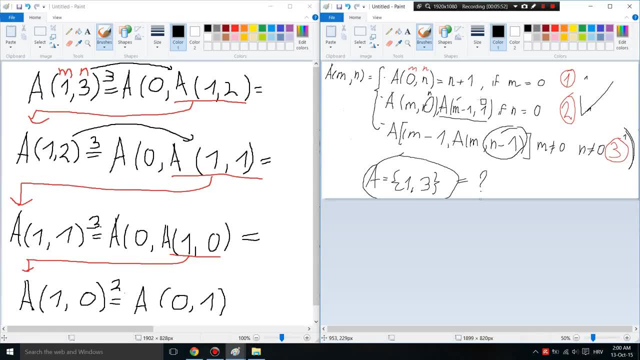 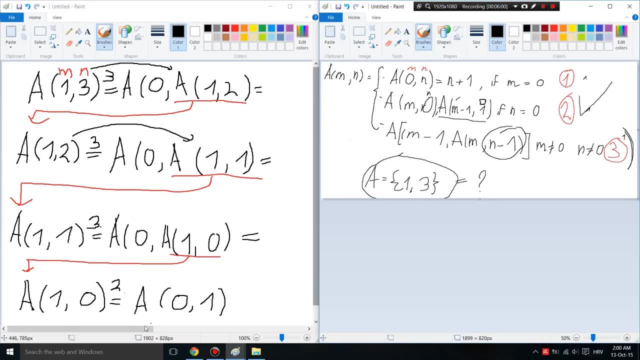 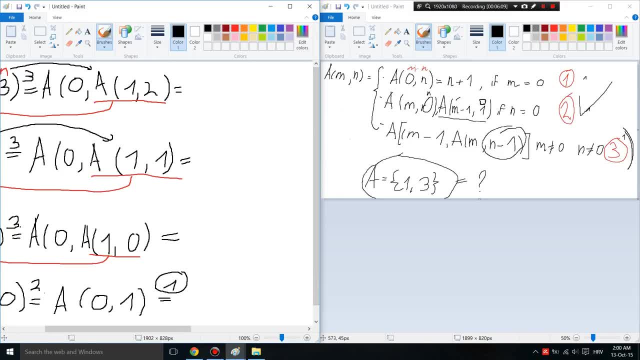 number one, and if it M is zero, and and it's something, but M is zero. so we, what we do is we add n plus one, so we go: one plus one equals two. now take this number two and we put it in this: a, but not this: